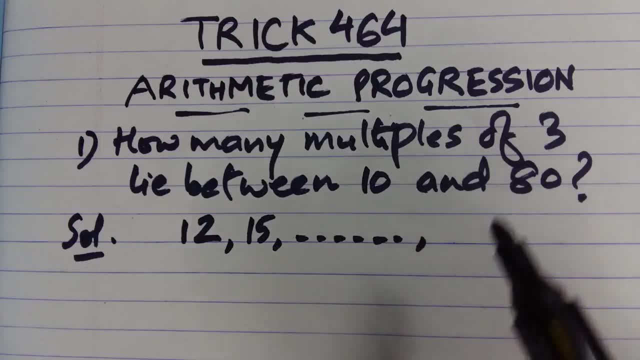 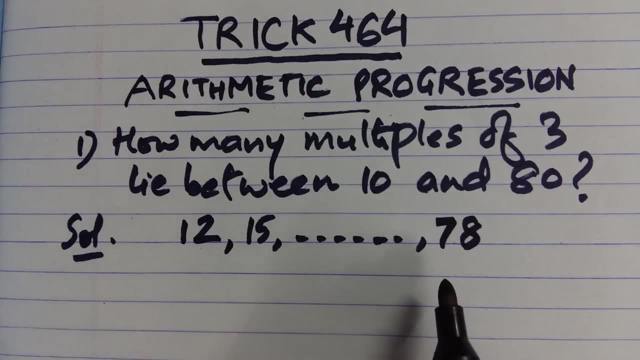 we need to find the one which is smaller than 80. So 81 minus 3 is 78. So our last number will be 78.. Now we need to count how many number are these? So for that you can use the formula for finding the value of n when first term, the difference. 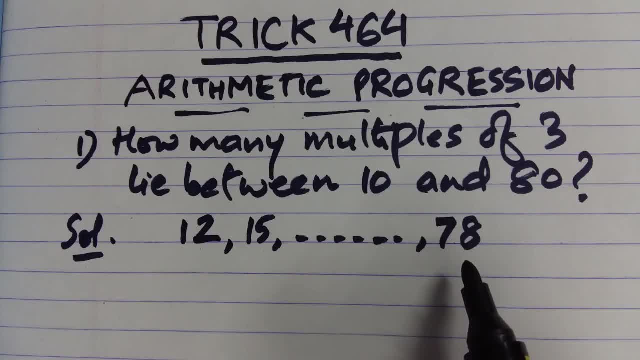 and the last term is given, But simultaneously I must tell you that this number is lowest, number is 12.. So the multiples 3,6,9, they are not included in these series. So if you would have taken these three numbers also, the series would have been starting with 3,, 6,, 9 and up to 78.. So what I have? 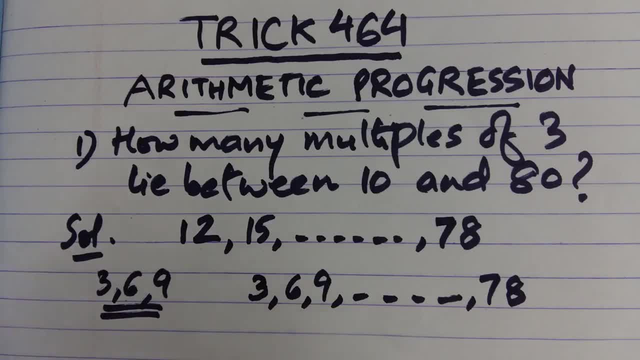 done is I have included the missing multiples here, And now you can see that all are multiples of 3.. So you can take 3 common and you are left with 3: ones are 3, 3, twos are 6, 3, threes: 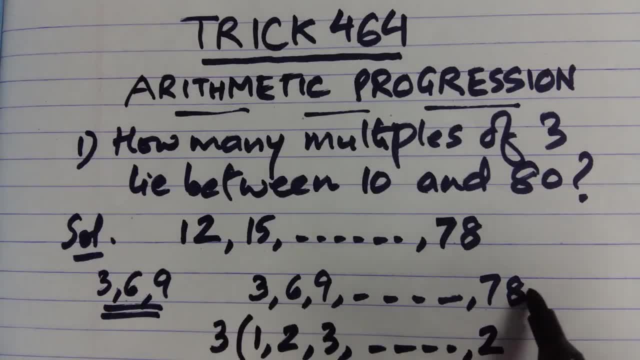 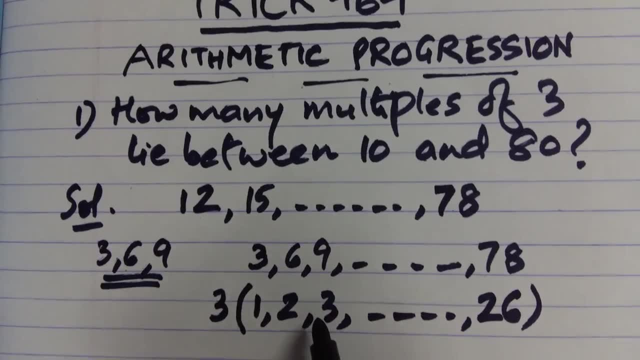 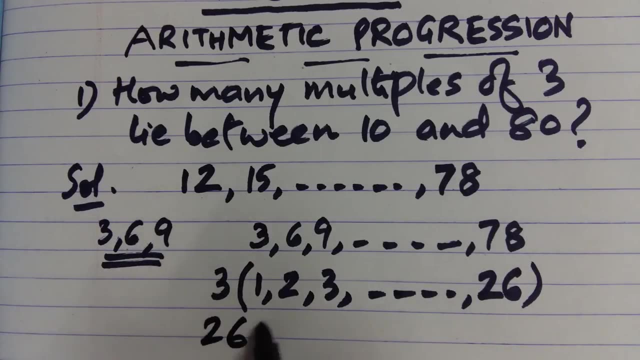 are 9, so on up to 3. twos are 6 and 18,, so 6, 26.. Now 1,, 2, 3, these are obviously natural numbers, So you don't need to count them. So these are 26 numbers, But since you included, 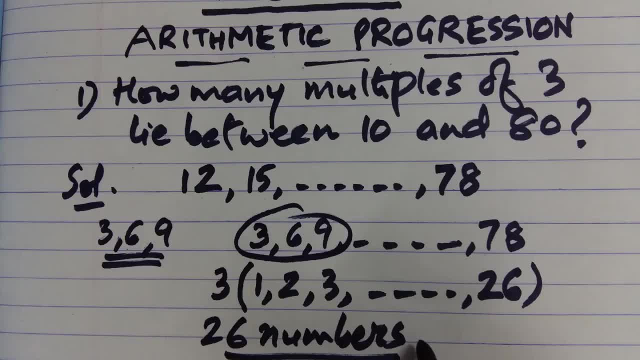 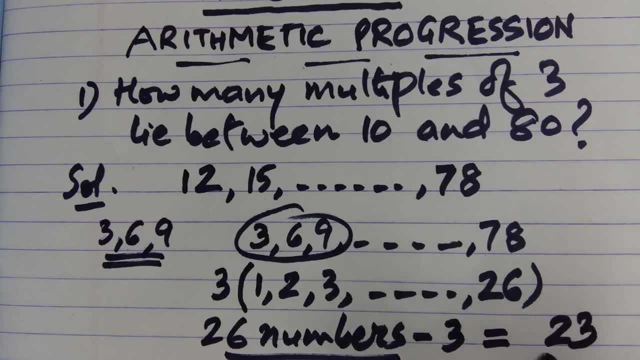 these 3 from your own side. so we need to subtract 3 numbers from this, So our answer will be 23.. So the trick here is to find out the missing numbers. Had it been a question number, we would have got the missing numbers. So we would have got the missing numbers. 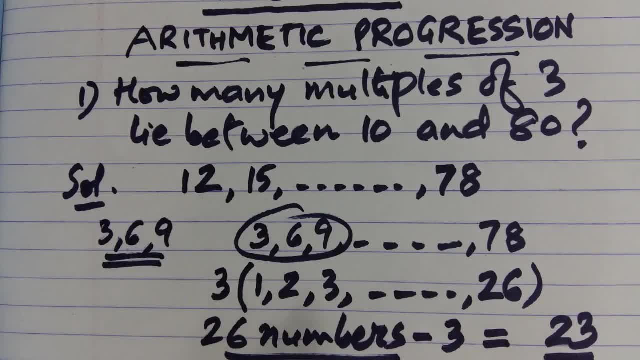 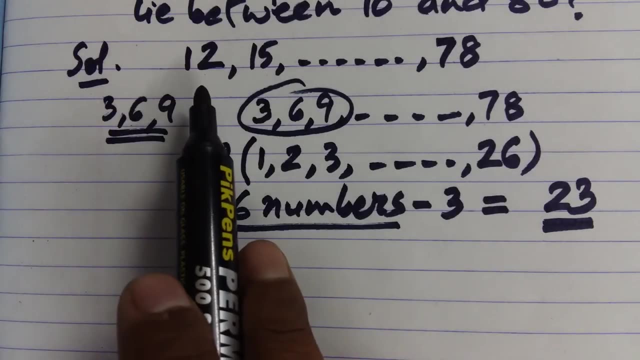 So we would have got the missing numbers. So we would have got the missing numbers. If you want to find the sum of all these numbers, then again it would have been very easy. If you want to find the sum of these 23 multiples, that is, 12,, 15, up to 78,, then you can use. 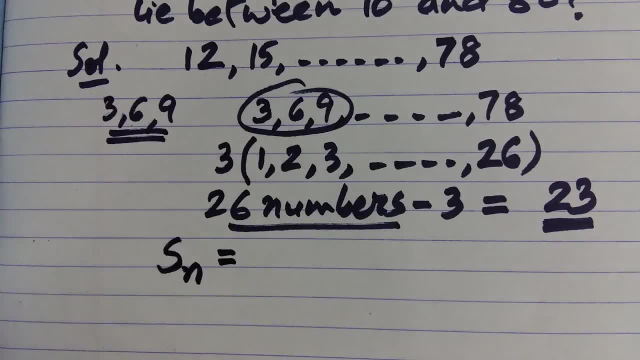 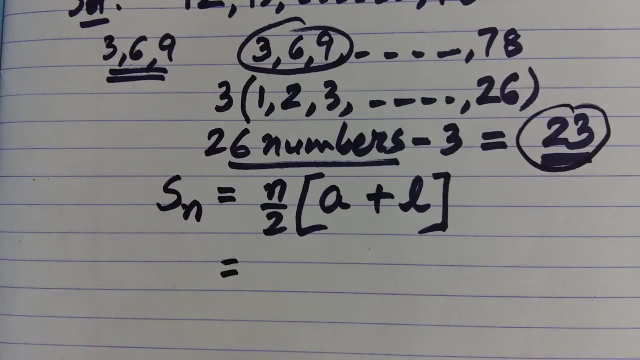 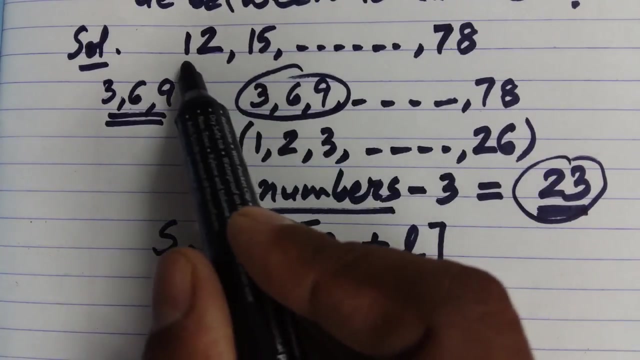 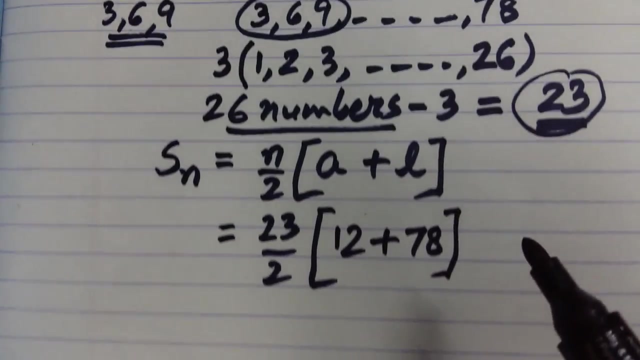 the formula for sum of n terms, which is n by 2. So n here is 23, because these are 23 numbers. So 23 by 2. And you can see in the series that the first term here is 12 and last term is 78. So 12 plus 78. This gives you 23 upon. 2 multiplied by 2.. So this is 23 by 2.. So n here is 23, because these are 23 numbers. So the result is that we got the missing numbers, So the answer here is 24.. So the result: here is 24 and 2 is held together by 90. There is no combination with 2 and 3. So 2 is a urt and 2 is aurt and 2 is to be cancel and 2 is to be multiplied and 3 is to be multiplied. 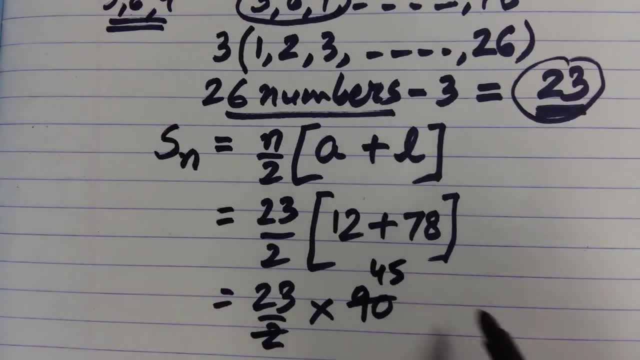 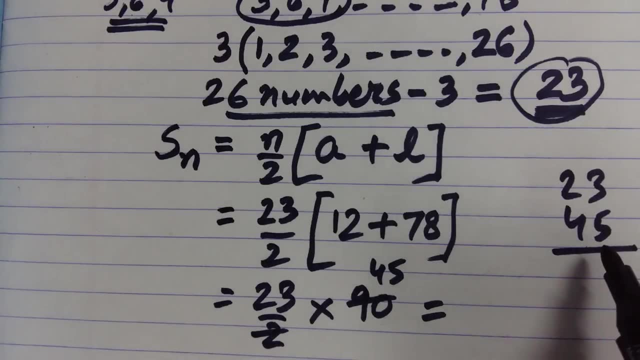 by 90. So 2 cancels 45 times, And all you need to do is to multiply 23 and 45 to get the final answer. You can use the Vedic method also here. 5 is a 15. So 1 curry, 5 2s are. 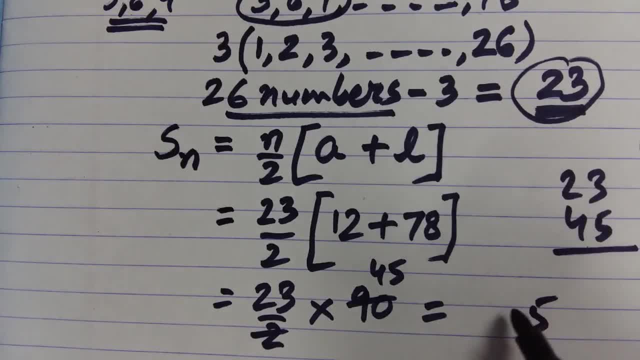 10 and 12, 22 plus 1, 23.. 3, 2 carry And 4: 2s are 10,, 4: 2s are 8 plus 2 is 10, so 1, 0, 3, 5 is the sum of all these numbers, So the results will be a 10.. So 5, 2s a 20.. 5, 2s, a. 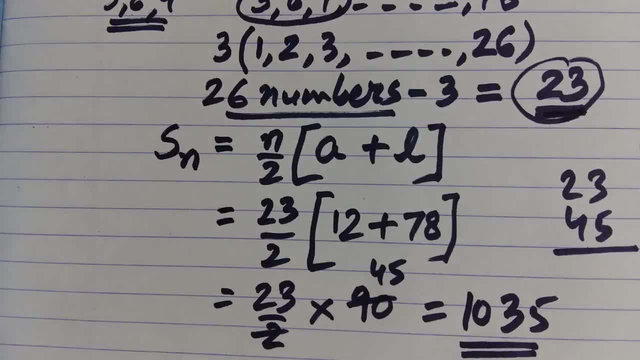 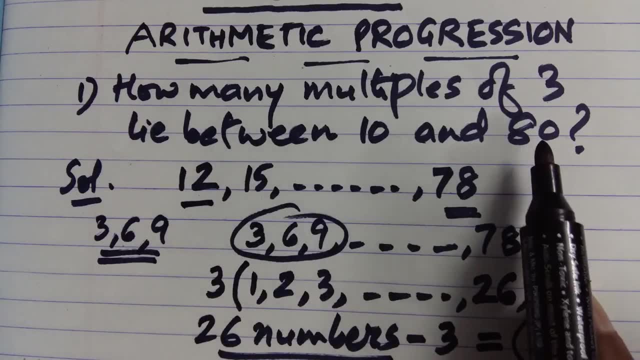 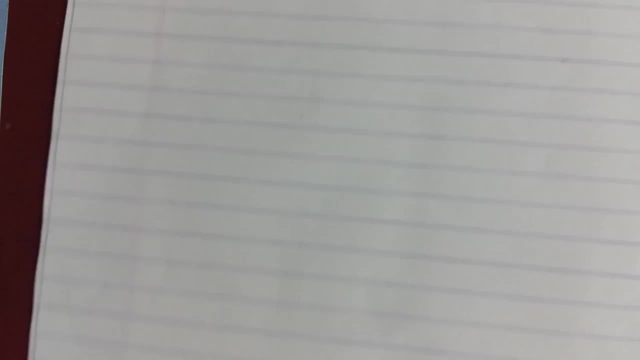 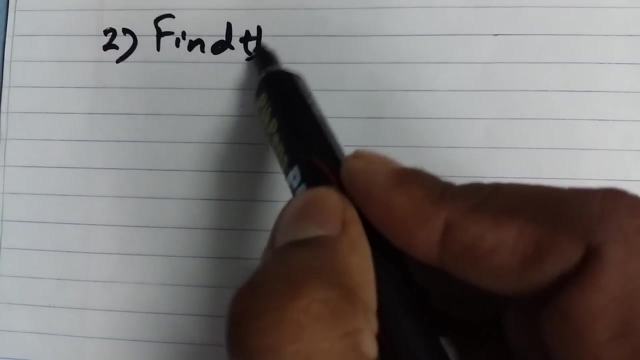 all these 23 numbers. So through this method we have found out how many multiples of 3 lie between 10 and 80 and we have found out their sum also. Let us have one more question for practice. This is question number 2.. Suppose we need to find the sum of all multiples. 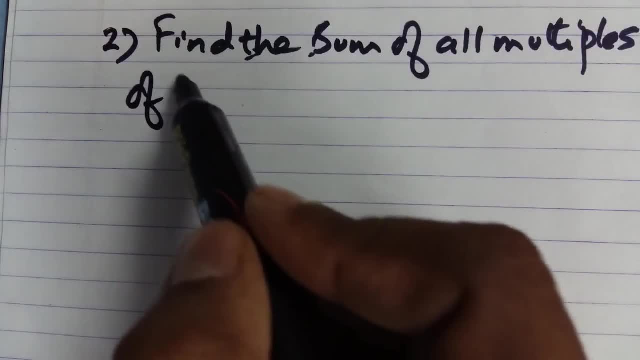 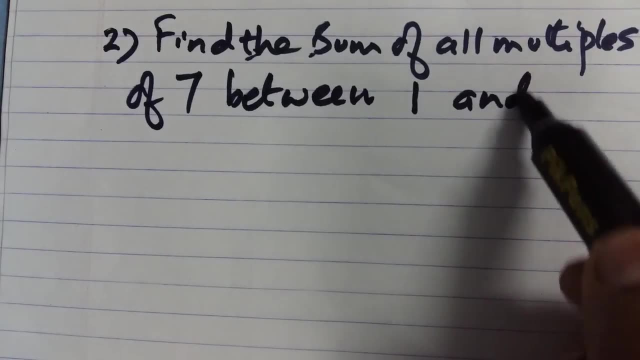 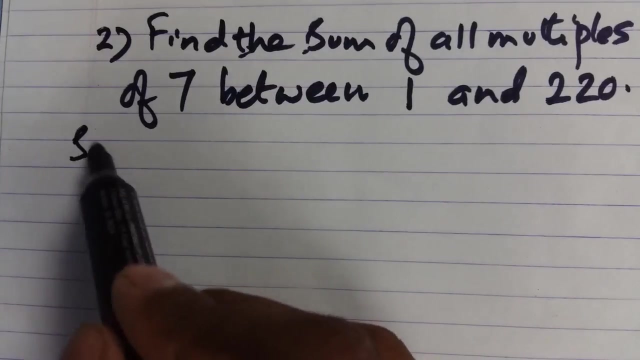 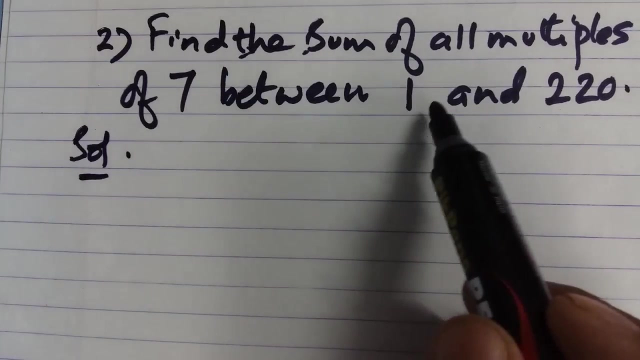 of 7, between 1 and, say, 220.. Now, first of all, we need to identify all the numbers which lie between 1 and 220 and which are multiples of 7.. So, obviously, the first multiple will be 7, followed by 14, it is a table of 7..